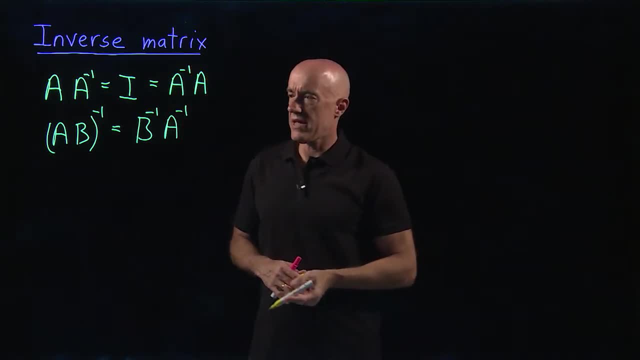 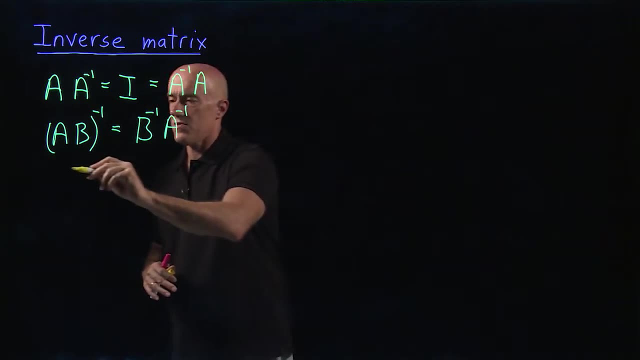 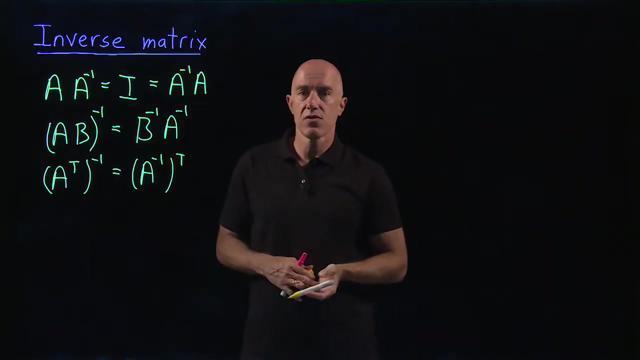 It's a relatively simple proof and I'm going to leave it to you guys for an exercise. The other one is what? if you're looking for the inverse of the transpose matrix, Okay, This is the inverse matrix: transpose. So that's another fact or theorem that I'll leave it. 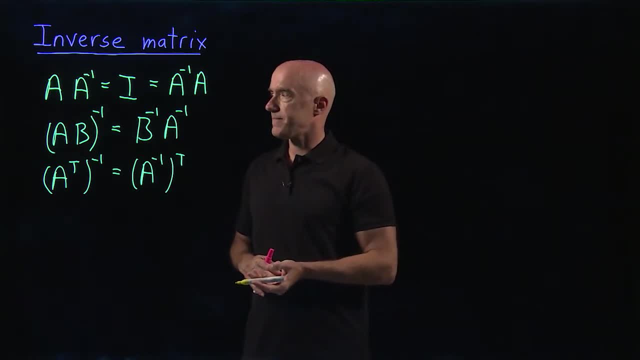 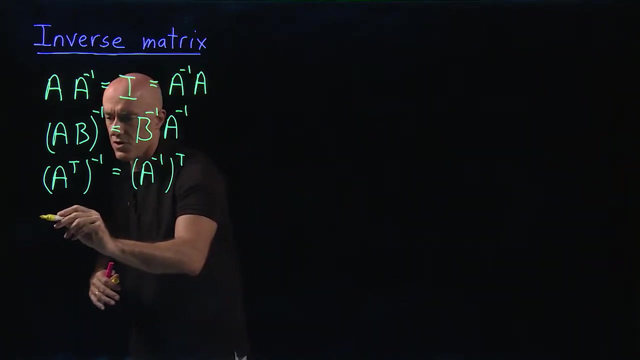 to you to do in the exercises. Okay, So what I want to do in this video is really compute the inverse of a two by two matrix, So we can set up some equations right. So let's look at the two by two matrix, So we're. 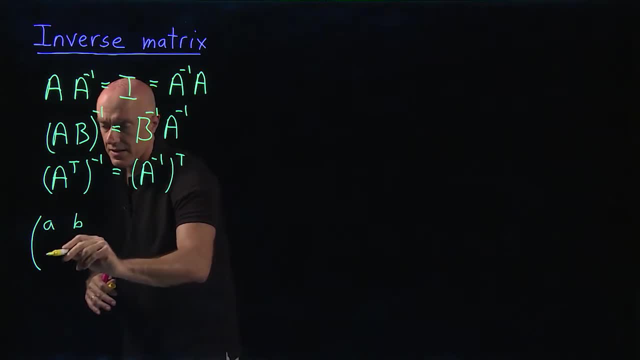 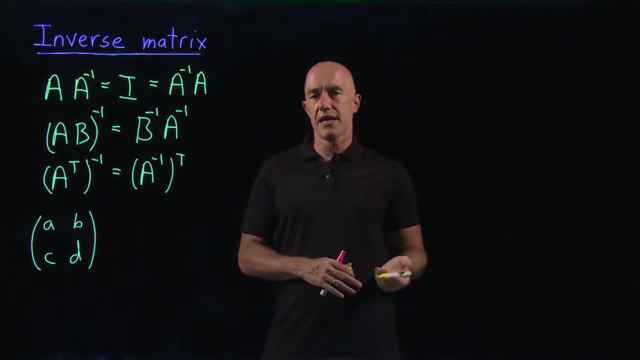 going to have a general two by two matrix- A, B, C, D- And I want to multiply this matrix by its inverse to get the identity matrix. So it's the inverse: is the matrix that we don't know. So that's going to be an unknown matrix. So let me write that as the first column. I'll 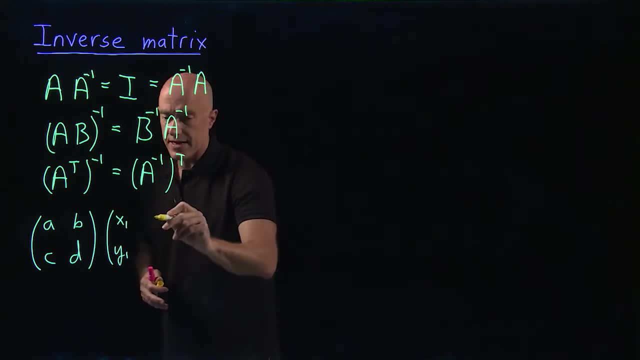 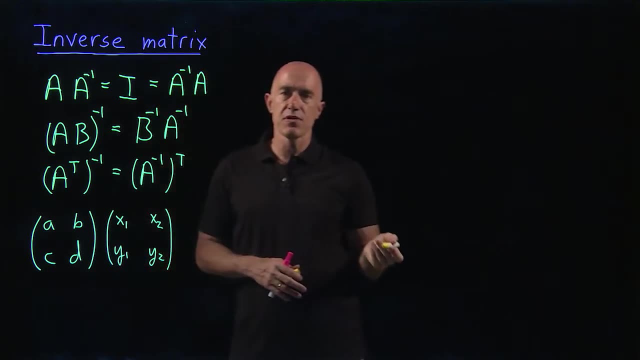 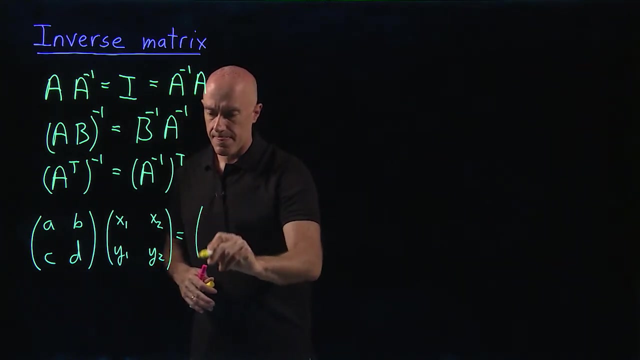 write as X1, Y1. And the second column I'll write as X2, Y2.. And that's supposed to be the identity matrix. So let me write that out. That's supposed to equal 1, 0, 0, 1.. 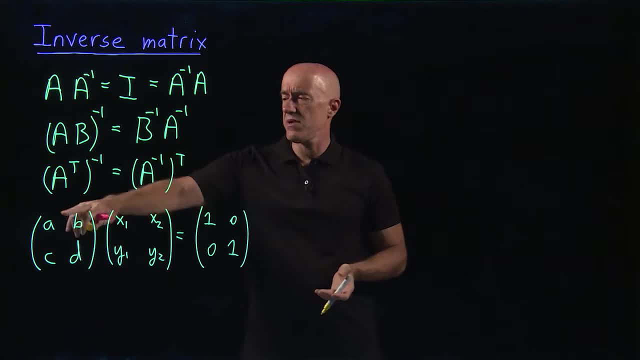 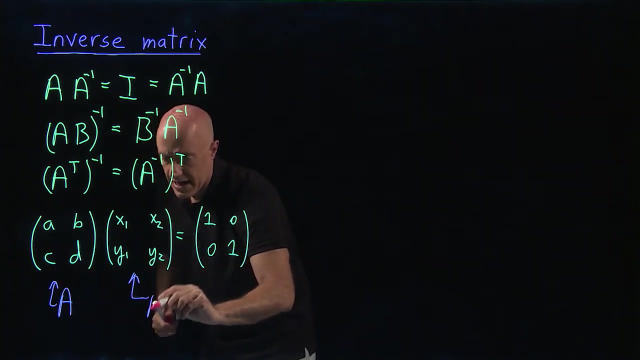 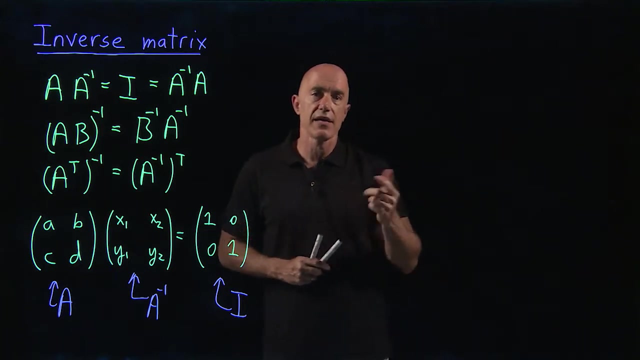 Okay, So the goal here is to determine what is the inverse of this two by two matrix, right? So I should make this clear: This one is our matrix A, This one is our matrix A inverse, And this one is the identity matrix. Okay, So we want to find A inverse. Okay, How do? 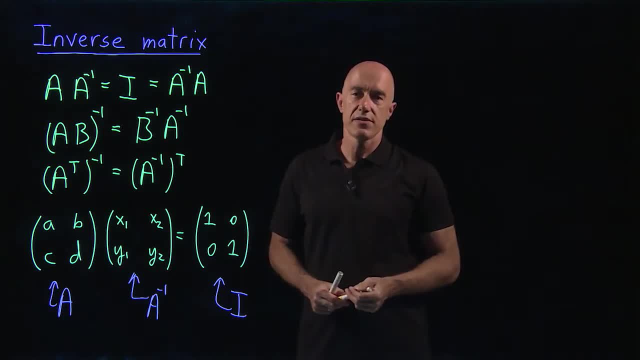 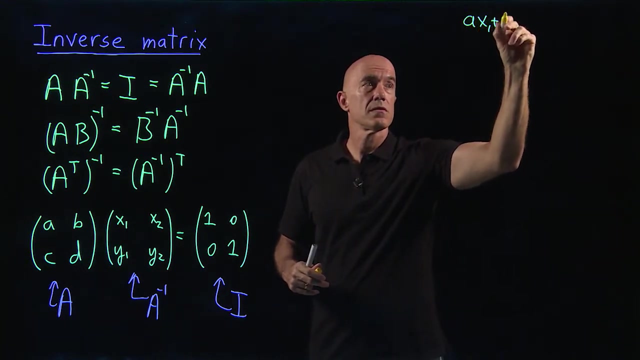 we do that. Okay, to write down equations. okay, If we write down the equations that this matrix product represents, then maybe we can solve for the unknowns. So let's see what is this. So we use matrix multiplication, So we have AX1 plus BY1.. AX1 plus BY1 is equal to 1, right. 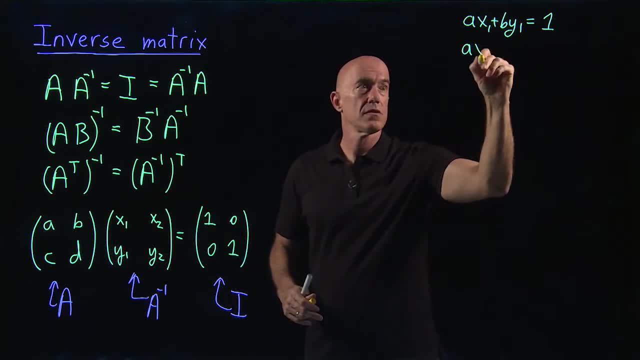 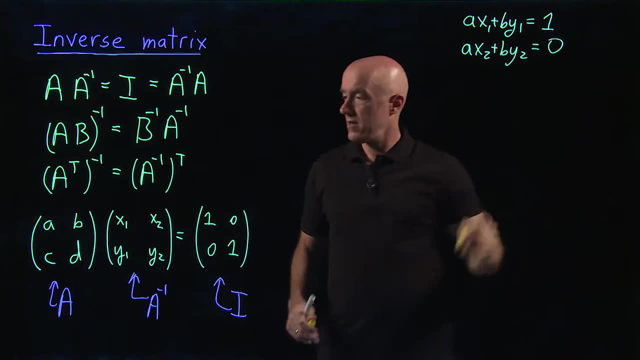 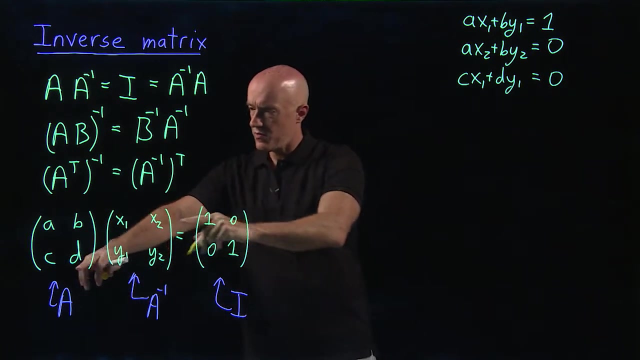 And then we have AX2 plus BY2.. And what is that equal to? That's equal to 0, right. Then, in the second row, we have CX1 plus DY1.. And that one is equal to 0.. And finally, we have 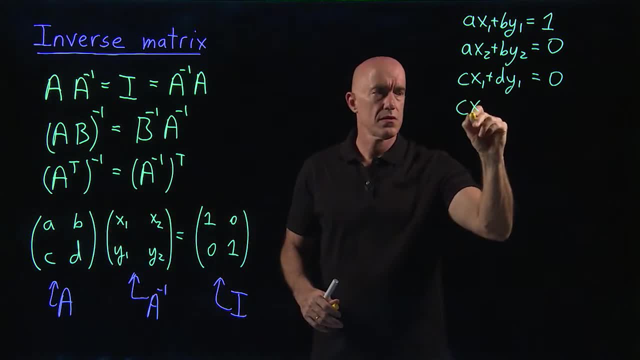 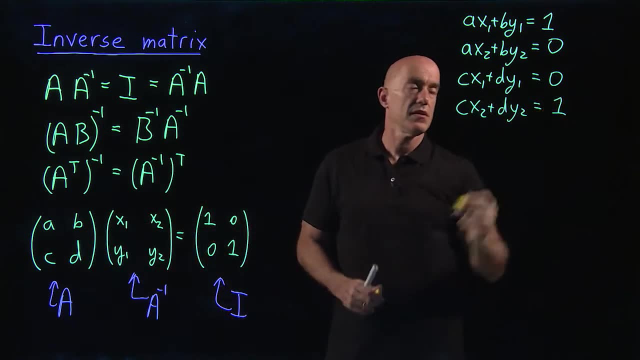 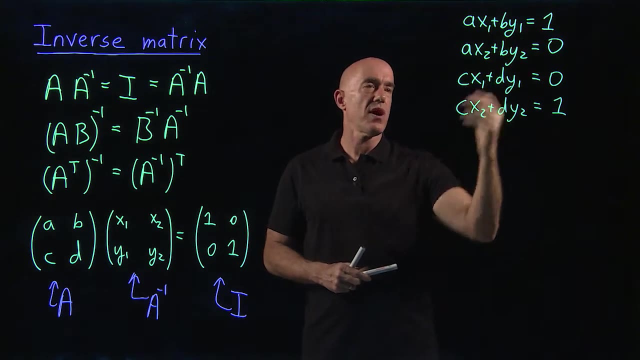 CX2 plus DY2.. And that's this last element here, which is 1.. Okay, We have four unknowns: X1, Y1, and X2, Y2.. And we have four equations. So you think we can solve for all the unknowns, okay. 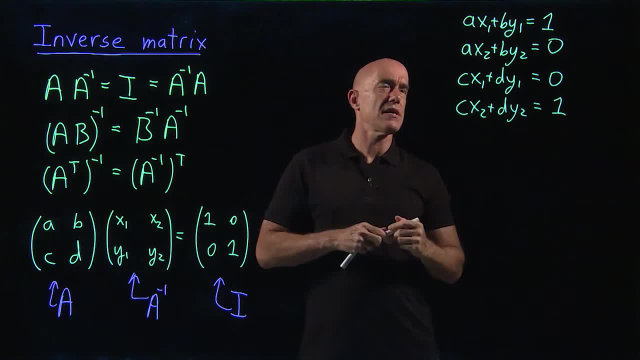 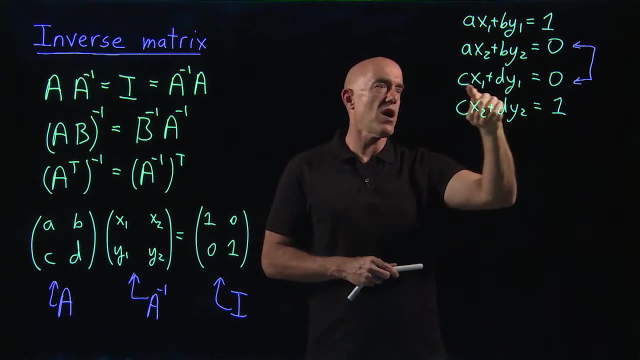 So how would we do that? I think the easiest way is to use these equations with the 0 on the right-hand side. Those are called homogenous equations And we can solve those equations for the Ys. So we can solve for Y1, we can solve for. 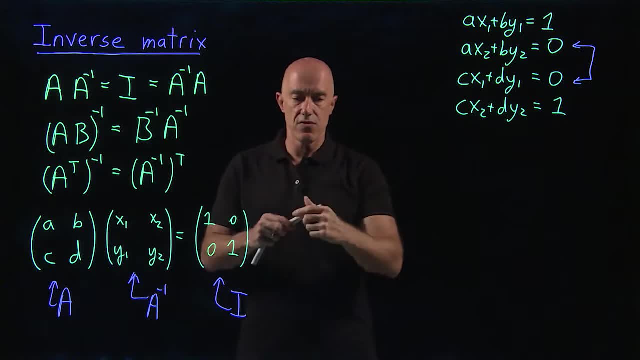 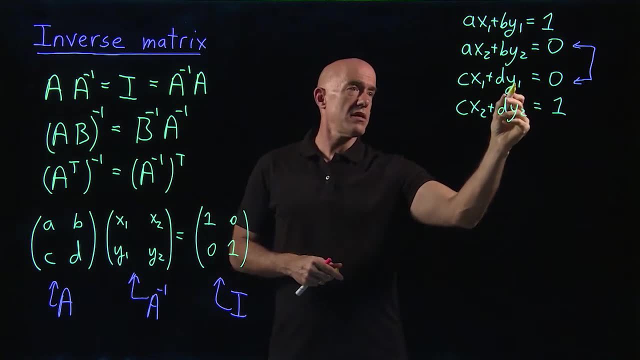 Y2.. So let's do that. I can put that over here: Cal for Y1 first, So DY1 equals minus CX1.. So then we solve for Y1.. So we get Y1, right, Minus CX1, divided by D, so minus CX2.. 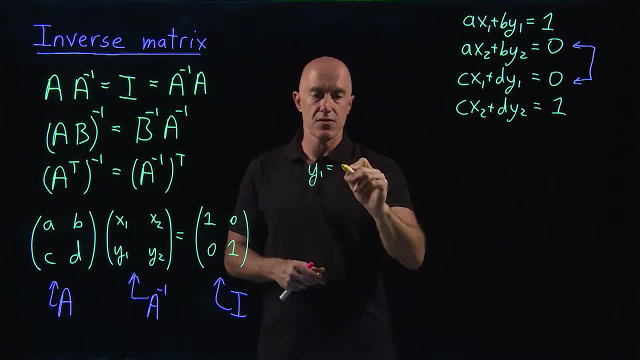 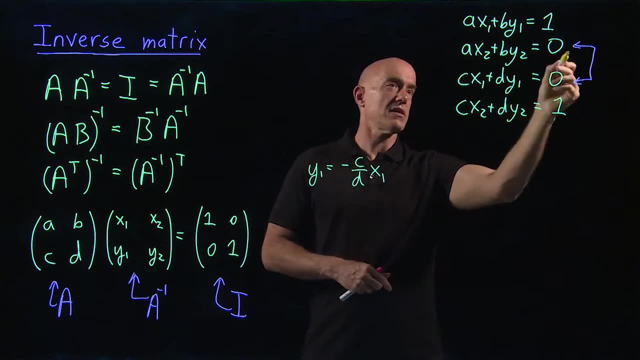 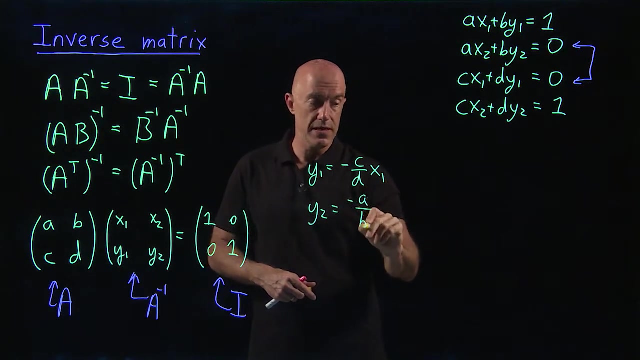 Can we process this? Yeah, yeah, c over d, x1, right. And the second equation we can solve for y2.. So we can subtract minus a, x2 and divide by b. so minus a over b. So this is: y2 equals minus a over b times x2, okay. 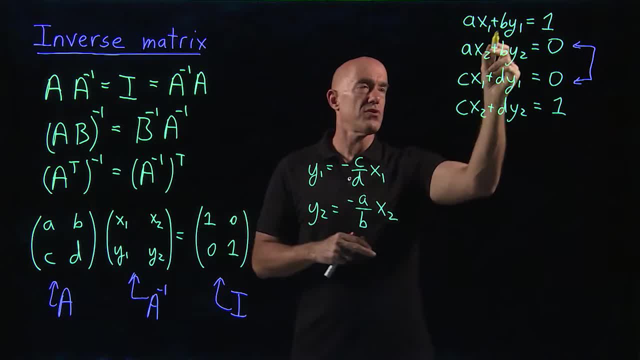 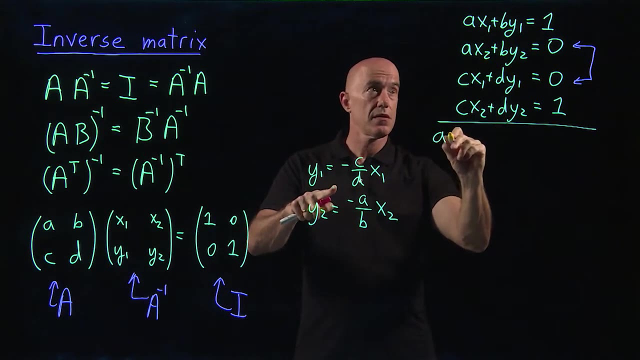 So we can eliminate y1 and y2 in favor of x1 and x2.. So now we go to the first equation. So let's see, we eliminate y1, so we get ax1 plus by1.. So by1,. so instead of plus we can use: 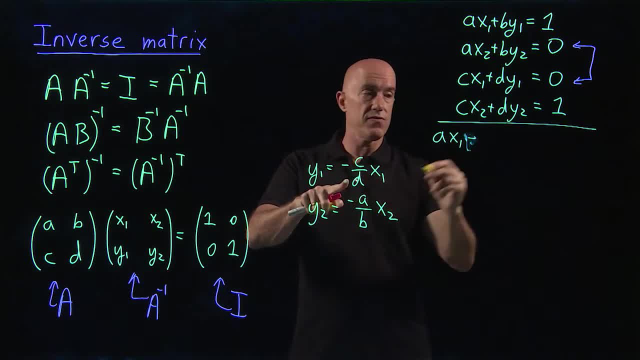 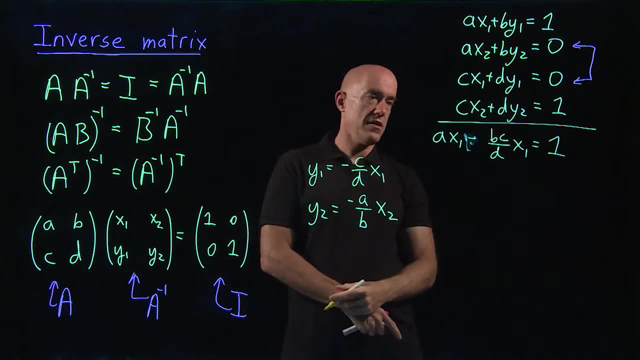 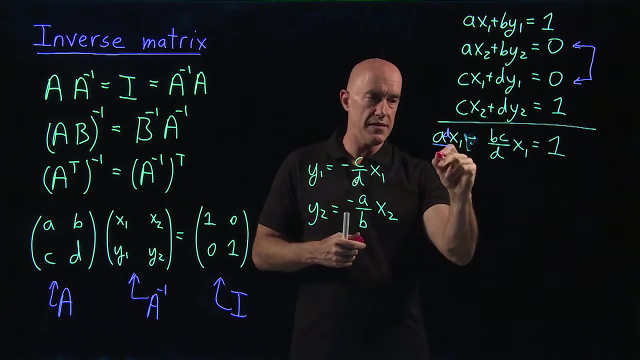 minus here minus bc over d. So x1 equals 1, right. We can multiply by d and divide by d right And then solve this equation for x1.. So you can factor out an x1, and then you have times ad minus bc divided. 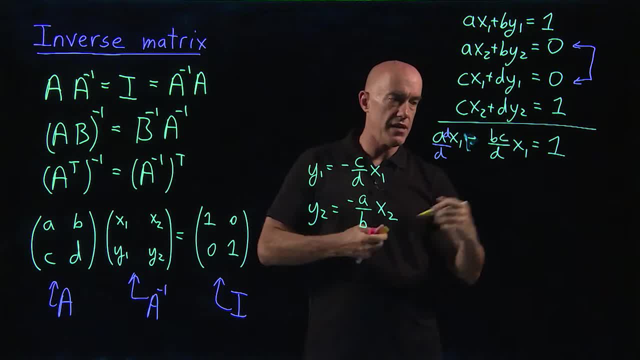 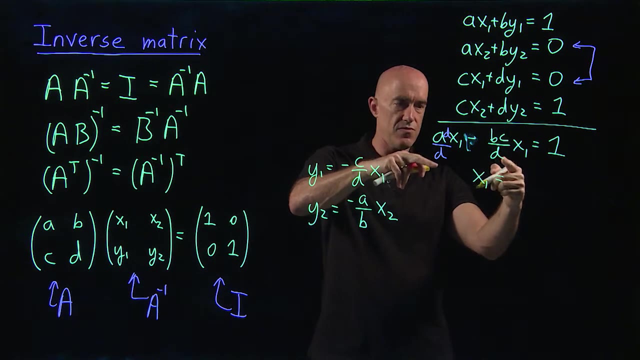 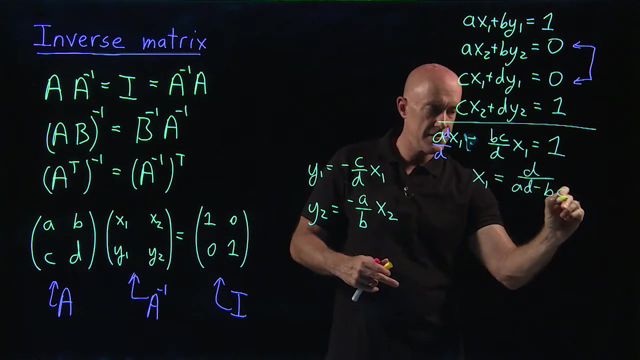 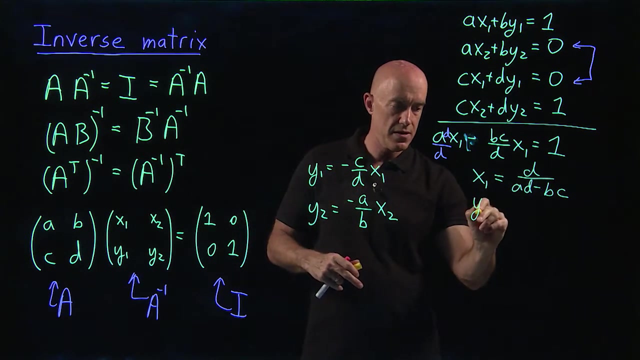 by d, and then you can bring that to the other side. So if you- let me skip some algebra stuff- So we can have x1 equal to, so we have ad minus bc over d and we flip that so that's d over ad minus bc. okay, So we've got x1.. If we've got x1, then we also have y1. So 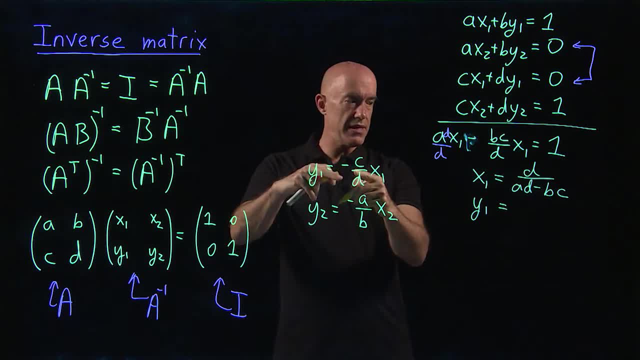 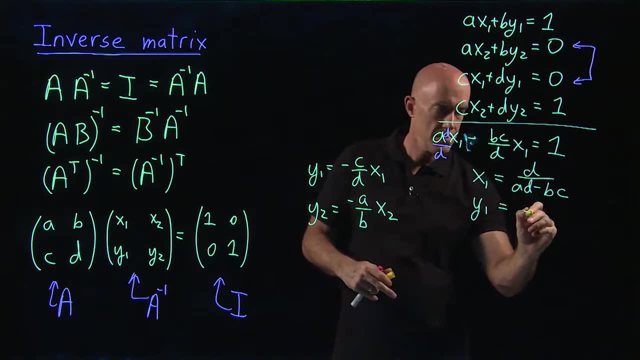 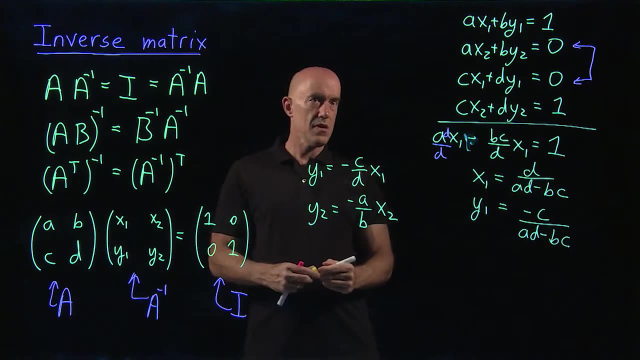 y1 is in terms of x1, so it's minus bc c over d x1, the d cancels, so it becomes minus c over ad, minus bc. okay, We're good. Now we need to find x2 and y2.. So we have y2 here in terms of x2, so now we need to. 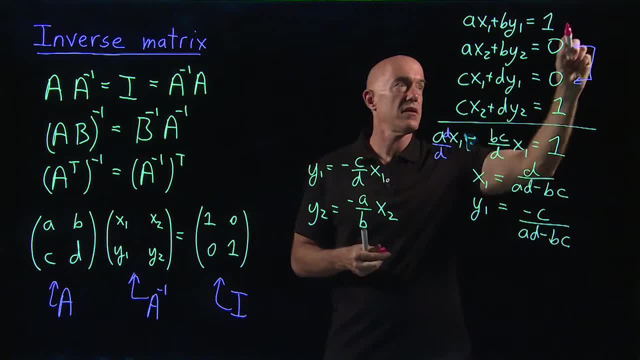 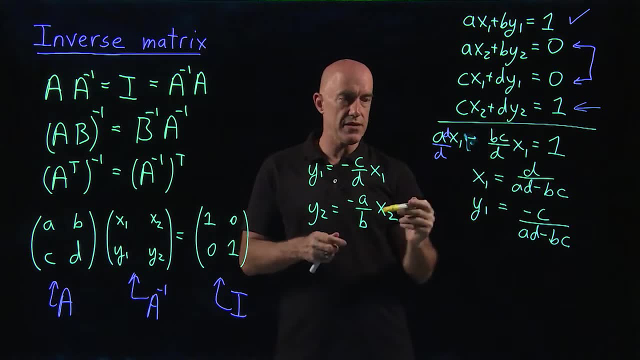 use the fourth equation. right? We just used the first equation, So now we need the fourth equation. So we substitute in y2.. Let me write it down here. So we have cx2 plus dy2, so that becomes minus ad over bx2 equal to 1.. Again, we do the same. 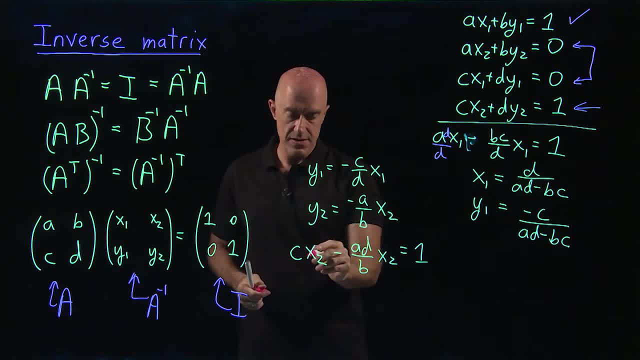 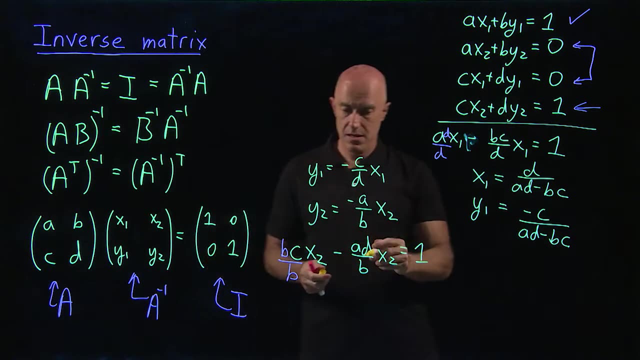 thing. So we have a b here in the denominator, So we have a bc and then a b, And then we can solve this for x2.. So we get x2.. Let me do it down here first. So we get: x2 equals b over bc minus ad. So bc minus ad is just. 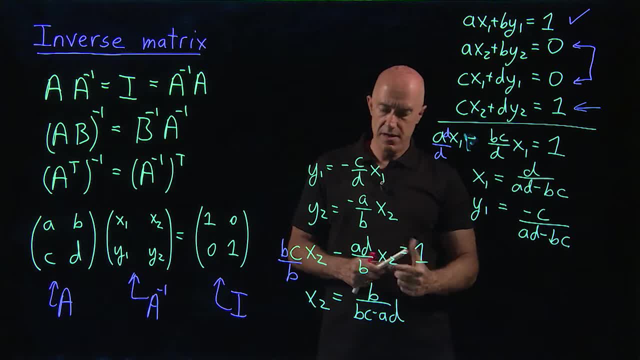 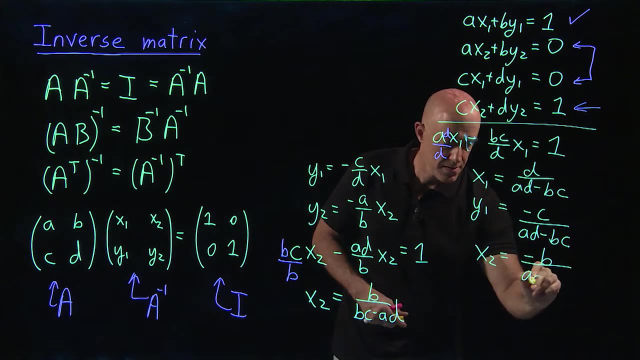 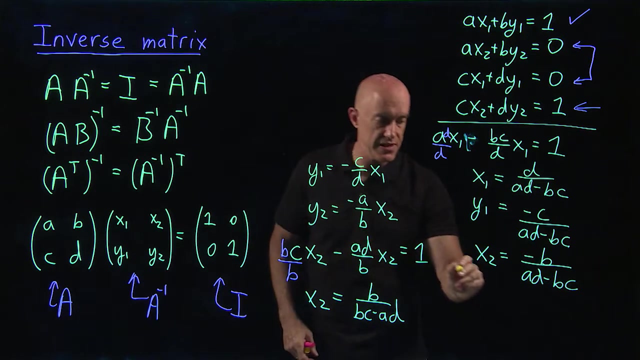 the negative, So we can write: x2 equals minus b over ad minus bc. Okay, we're almost done, We have x2, so now we just need y2.. So y2 is equal to x2 over ad minus bc. Okay, we're almost done, We have x2, so now we just need y2.. So y2 is equal to x2 over ad minus bc. 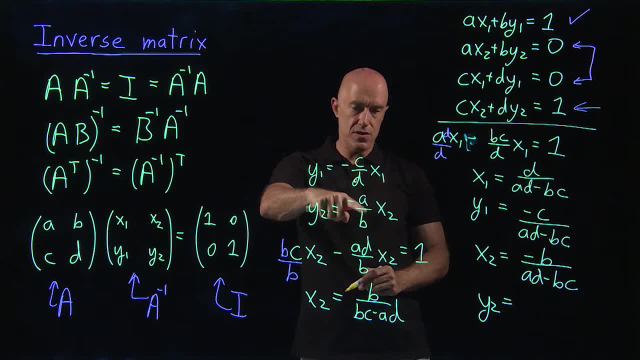 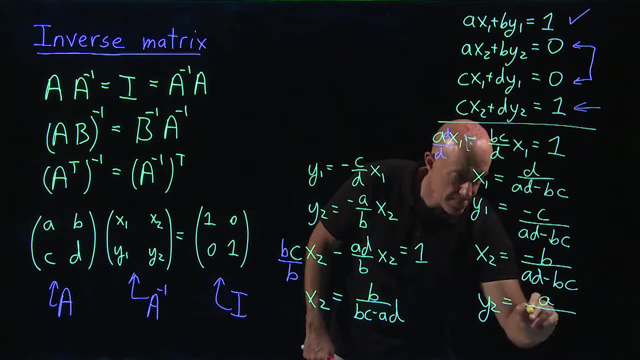 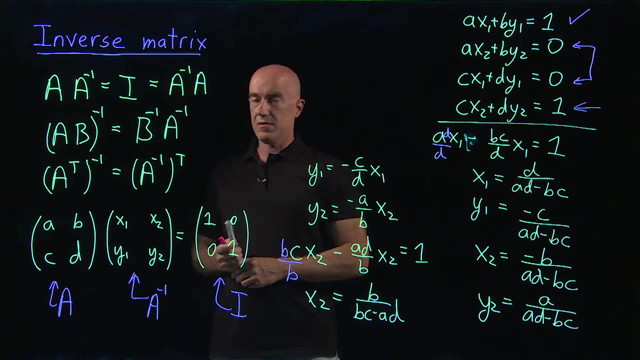 Minus a over bx2.. So the minus signs cancel. That becomes then a over ad minus bc. Okay, so we've got the result. So let me put it here. I'll use a different color, so you see that. So sorry, I'm going to write on my face, Maybe a little bit lower, So we have a inverse then. 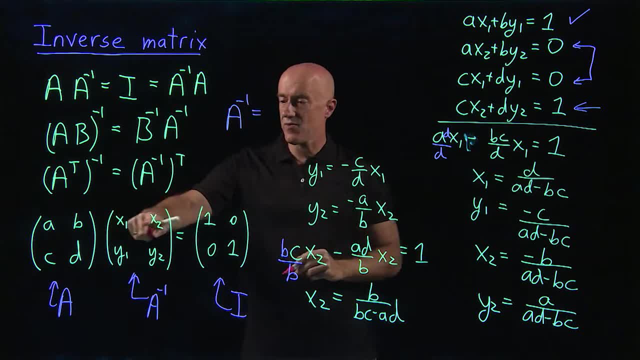 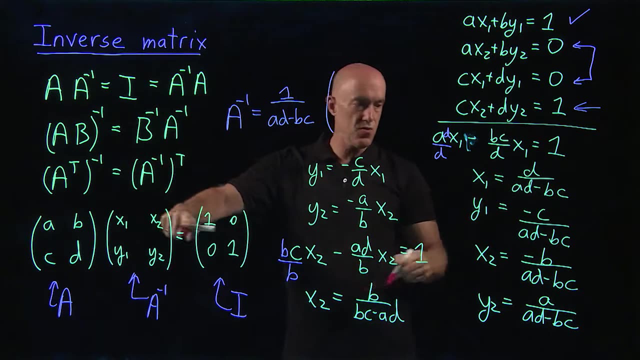 Okay, so what is a inverse? So x1, x2.. So there's always a 1 over ad minus bc, So 1 over ad minus bc, And then we have the matrix. The matrix is x1, x2.. So d minus b, And then we have y1, y2.. So we have minus ca. 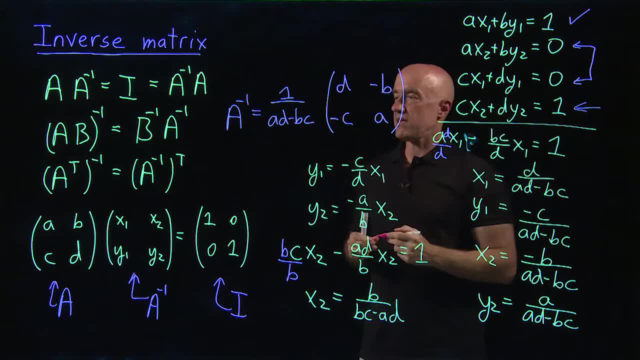 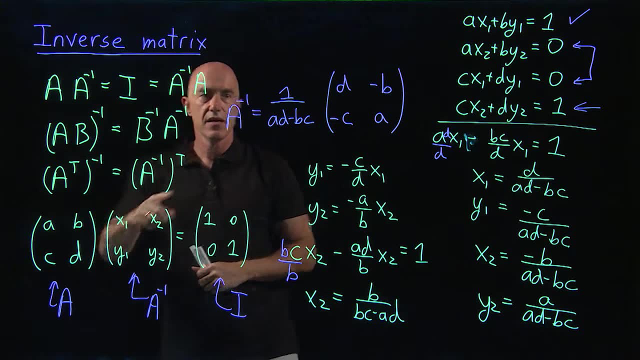 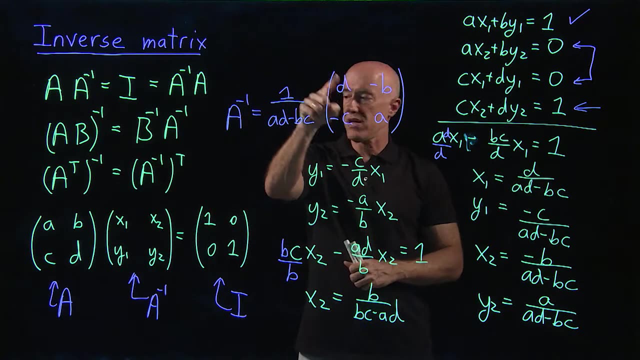 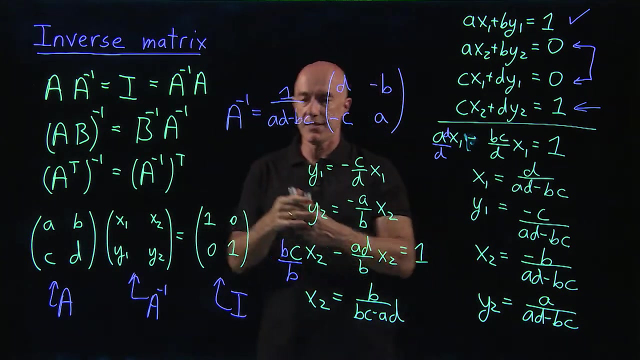 Okay, that's the inverse matrix, So interesting. a, b, c, d, The inverse of that is 1 over ad minus bc, And then the matrix itself, the diagonal element switch. So we have da, And then we just negate the off-diagonal elements minus b and minus c. 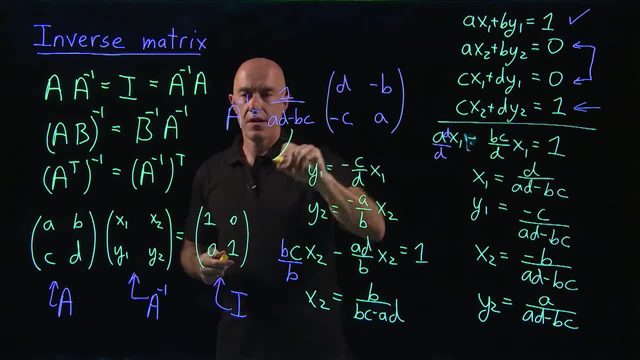 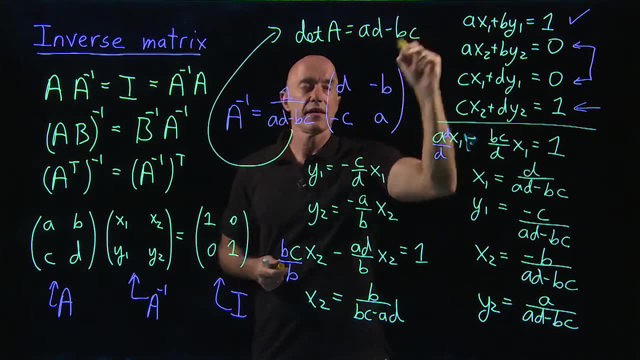 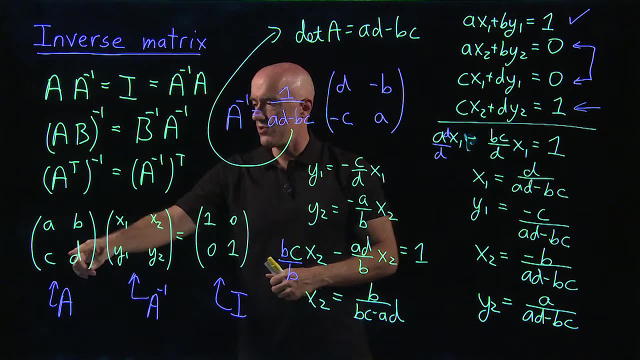 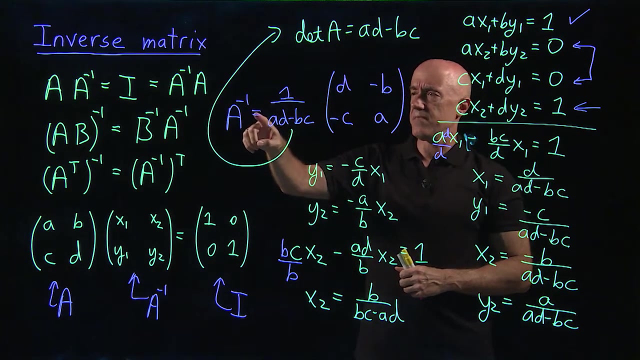 This piece here. ad minus bc is what we call. the determinant of a is ad minus bc, And that's for a 2 by 2 matrix. So that is this 2 by 2 matrix. The determinant is ad minus bc. And the interesting thing here is that if ad minus bc equals 0, you're dividing by 0.. So there is no inverse matrix.